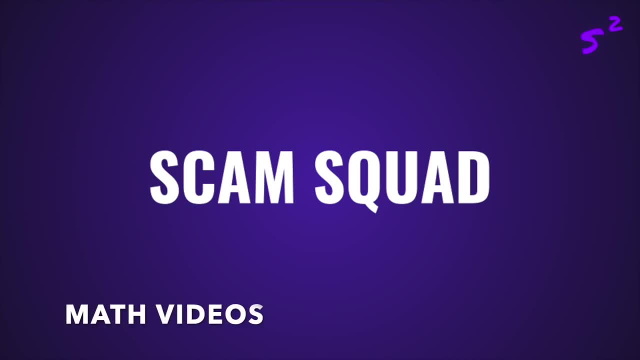 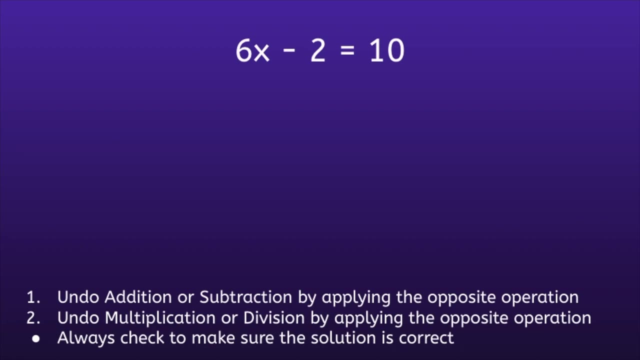 Example number one: 6x minus 2 is equal to 10.. The first step to solving a two-step equation is to undo addition or subtraction by applying the opposite operation. So if we look at the equation, we can see that there is subtraction And on the side with the x they are subtracting. 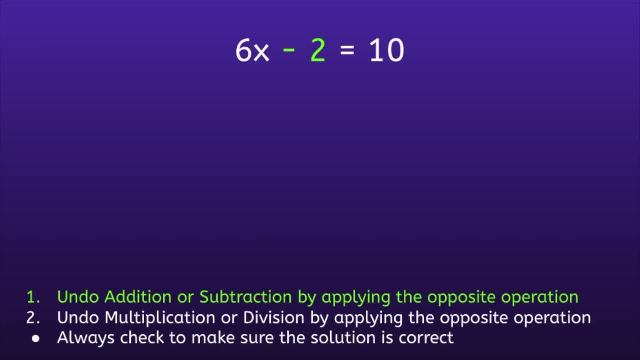 2.. So we want to do the opposite operation of that, and the opposite of subtracting 2 is adding 2.. And we're going to apply that on both sides of the equal sign. If we focus in on the left, we have a negative 2 plus positive 2.. Since those are opposite numbers, 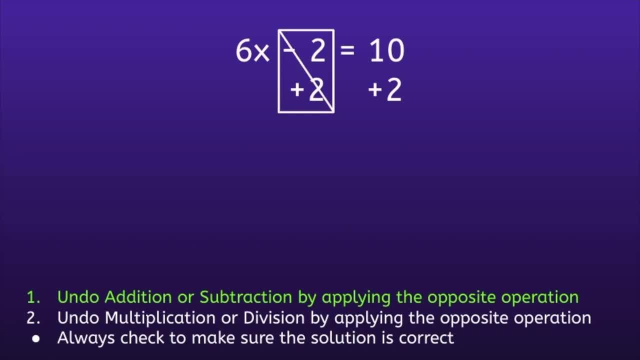 they will cancel out and equal 0,, which leaves me with 6x on the left side, And if I focus on the right side, I have 10 plus 2.. And 10 plus 2 is equal to 12.. Moving on to step two, Undo. 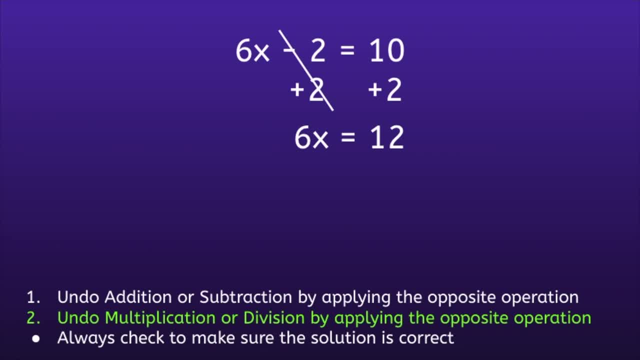 multiplication or division by applying the opposite operation. In this one, we have a number in front of the variable. This is called a coefficient. A coefficient is a number being a variable. So we want to do the opposite of multiplying by 6, which is dividing by. 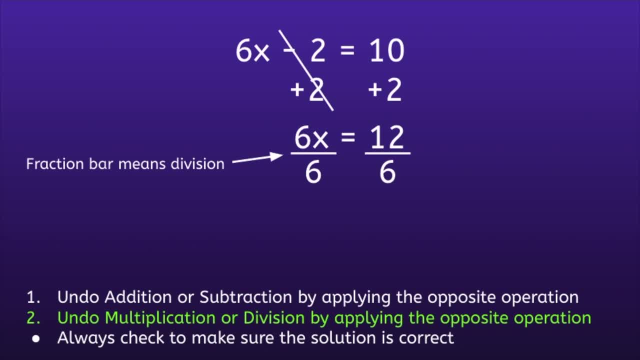 6. And that fraction bar in the middle means division. So if we focus on the left side, we have 6x divided by 6. And 6 divided by 6 is equal to 1.. So that will leave us with. 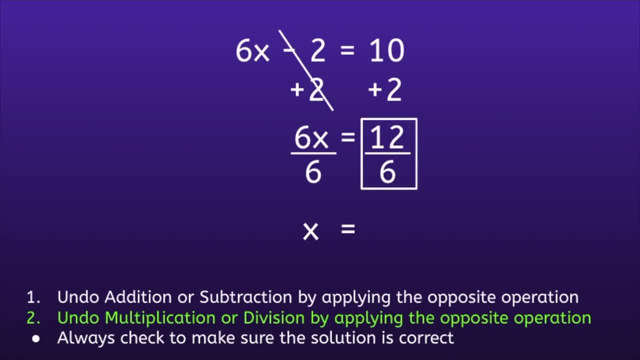 one x or just x. And if we focus on the right side, we have 12 divided by 6.. And 12 divided by 6 is equal to 2.. So we have our solution: x is equal to 2. But we're not done quite. 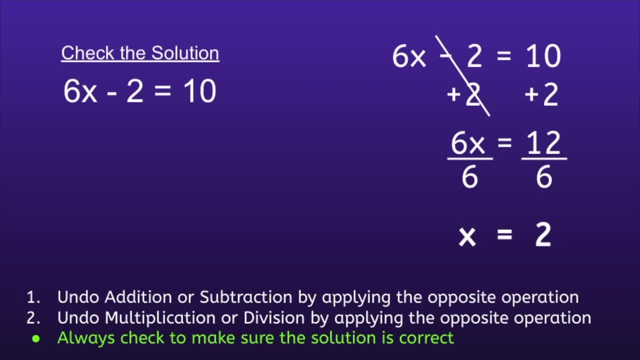 yet, because we always want to check to make sure our solution is correct. So we can rewrite the original equation: 6x minus 2 is equal to 10, and replace the x with our answer, which our answer was 2, so I'll replace that x with a 2.. And remember, since that 6 was 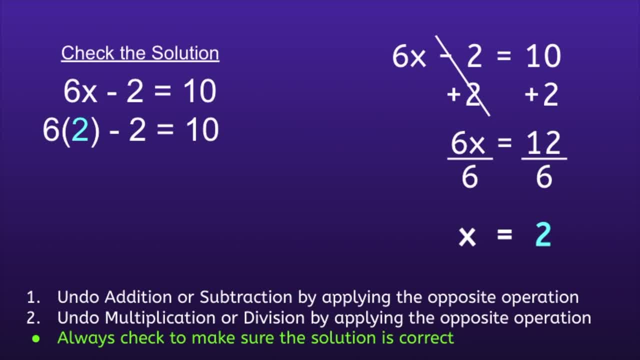 in front of the x. that means that we are multiplying. So we have: 6 times 2 minus 2 is equal to 10.. And we want to see if those are equal on both sides of the equal sign. Well, 6 times 2 is 12.. 12 minus 2 is equal to 10.. So since 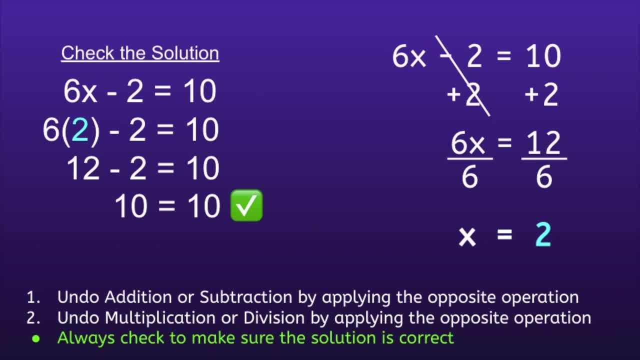 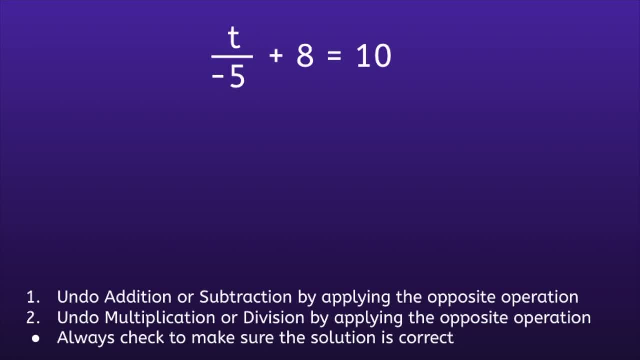 both sides are equal, we know our solution is correct. So the final answer is: x is equal to 2.. Example number 2. t over negative 5 plus 8 is equal to 10.. Step 1. Let's do addition or subtraction by applying the opposite operation In this one. we can. 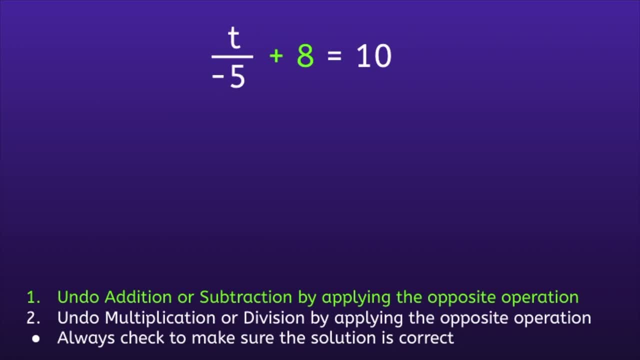 see that we have plus 8.. And the opposite of a plus 8 is a minus 8.. And we're going to do that to both sides of the equal sign. If we focus on the left, positive 8 minus 8 cancels out, so we're left with t over negative 5. And on the right side we have 10 minus. 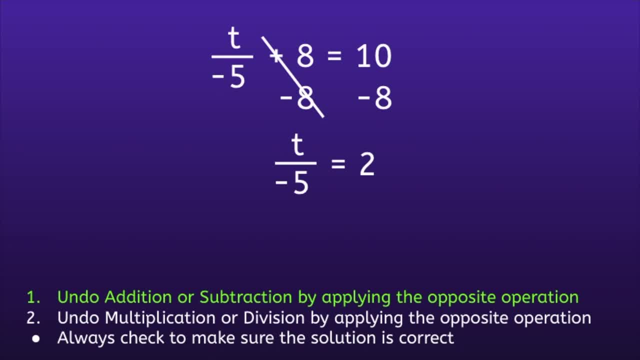 8. And 10 minus 8 is equal to 10.. So we're left with: 10 minus 8 is equal to 2.. This moves us on to step number 2.. Undo multiplication or division by applying the opposite operation. 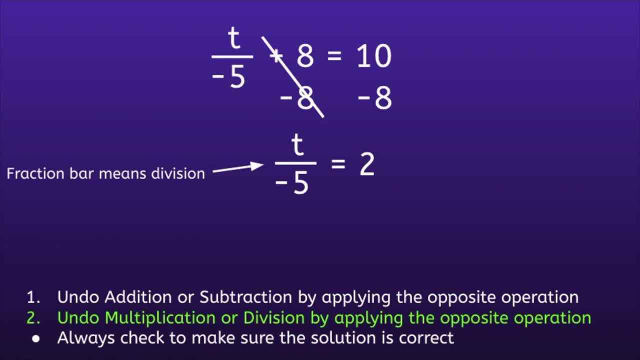 Well, if you remember from the last one, the fraction bar means division. So we are dividing t by negative 5.. So what's the opposite of dividing by negative 5? Multiplying by negative 5.. If we focus in on the left, first thing we're going to want to do is change that negative. 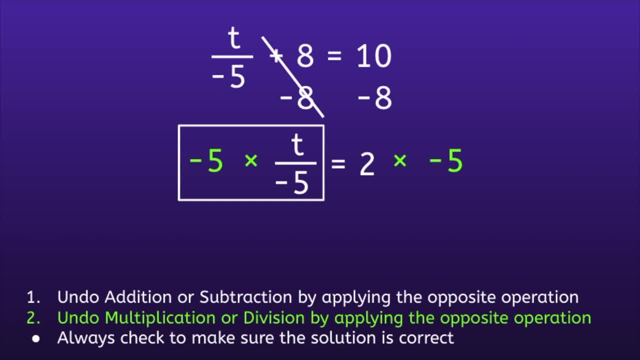 5 into a fraction. And we can turn any whole number, no matter if it's positive or negative, into a fraction by giving it the denominator of 1.. We also want to notice that in front of that t there's an invisible number, And that invisible number is a 1.. So if we pull 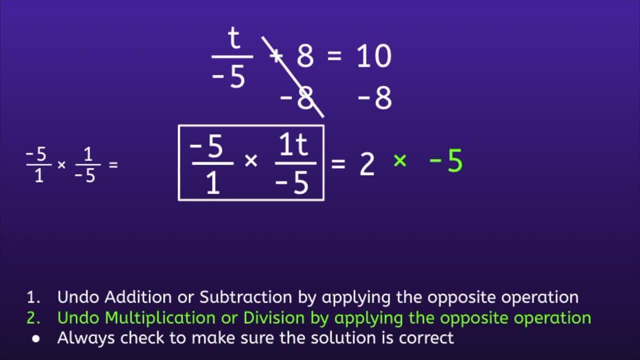 out just the numbers and ignore the t. we have negative 5 over 1 times 1 over negative 5. And these fractions are called reciprocals because they're the same except for the numerator and denominator are switched, And any time you multiply reciprocals, you will always.